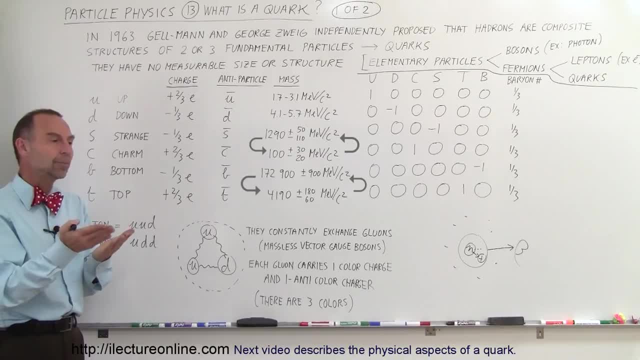 So the concept was that quarks would make up hadrons, which of course make up the baryons and the mesons, the heavy particles making up the mass of the universe. And so they surmised that the heavy particles, the baryons, probably had three of them in. 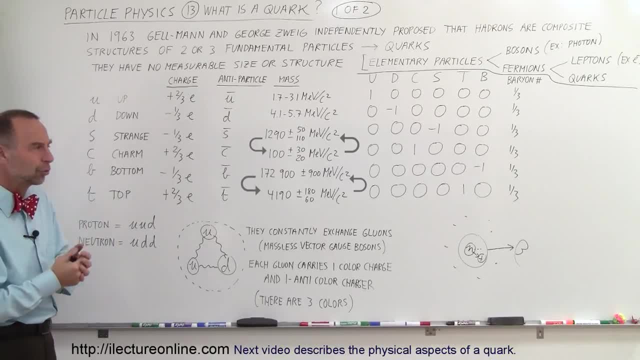 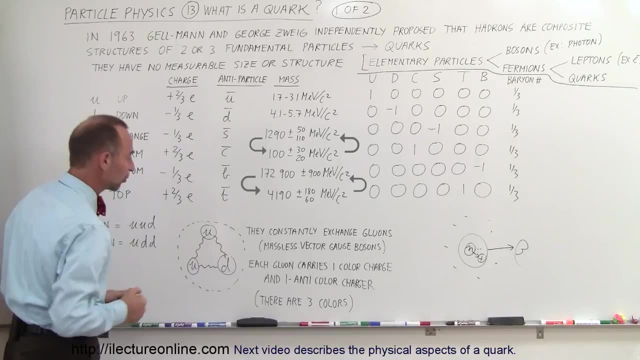 there, and that the mesons, the lighter particles, So the middle heavy particles, would have two of these quarks in there, And so the concept was that we would have a proton or neutron consisting of three quarks, and that the type of quarks would then dictate whether or not those particles would have. 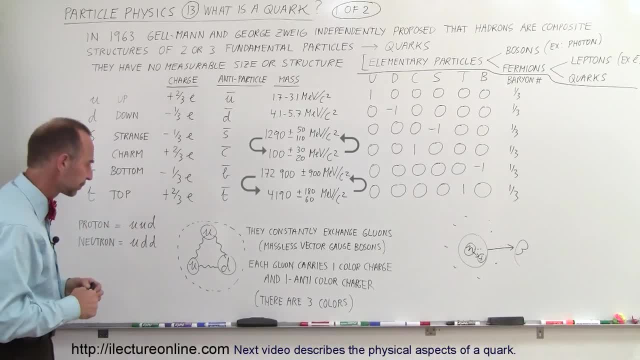 a positive charge, would be neutral or would have a negative charge, And so it was then surmised that there were different kinds of quarks, and so they started studying this and trying to figure out how many different kinds of quarks there actually. 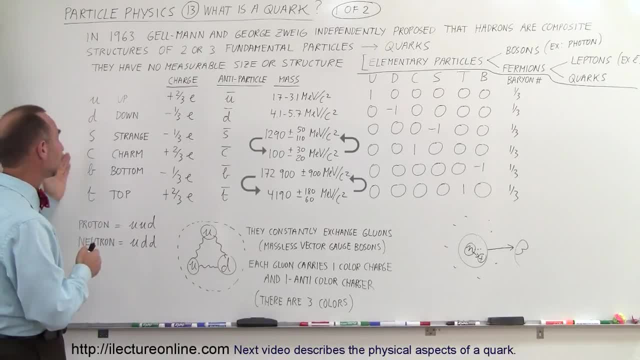 were, And it turns out at this point there are six different quarks that are being discovered, And so those are what we call the up quark, the down quark, the strange quark, the charm quark, the bottom quark and the top quark and the associated antiparticles. 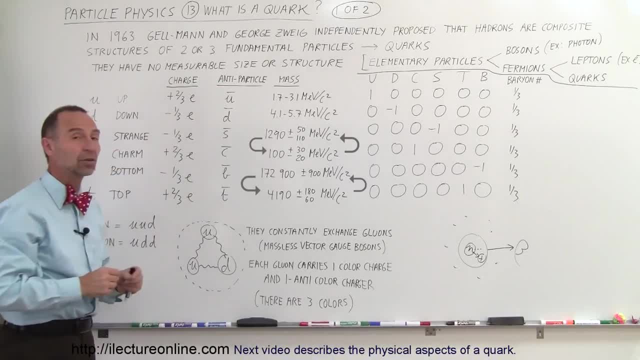 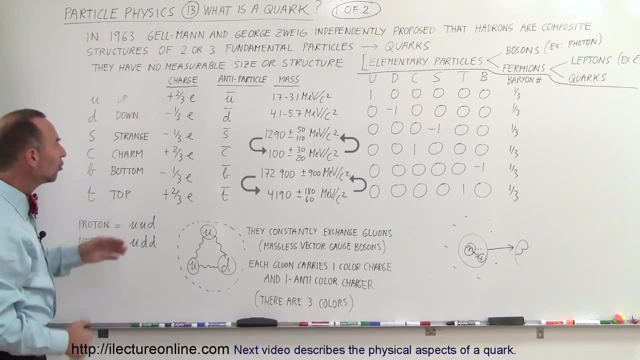 So for those six quarks there are six associated antiparticles that have the same mass but the opposite charge, just like an electron that has an antiparticle called a positron. They also discovered that these particles either had a positive, two-thirds charge, positive. 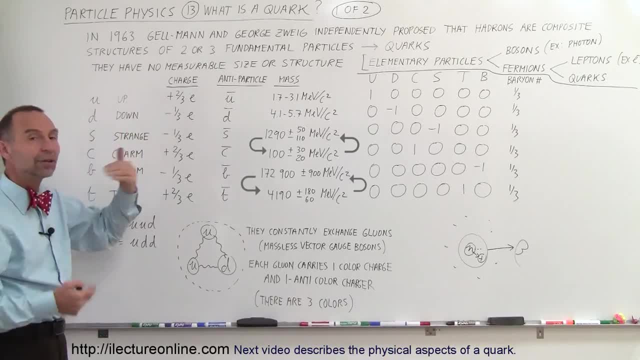 two-thirds of an electron charge over a negative one-third of an electron charge. And when I say electron charge, I mean the absolute value of the charge, not the actual sign. So there's an electron charge which is 1.6 times 10 to the minus 19 coulombs. 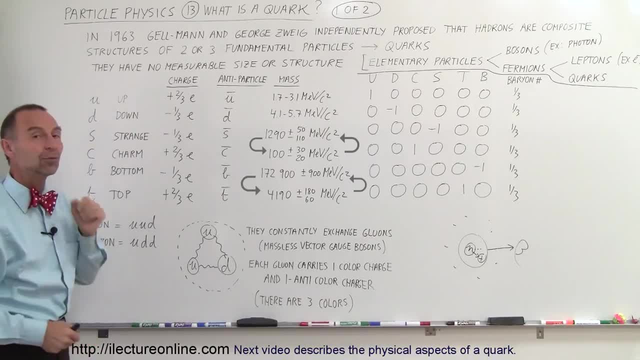 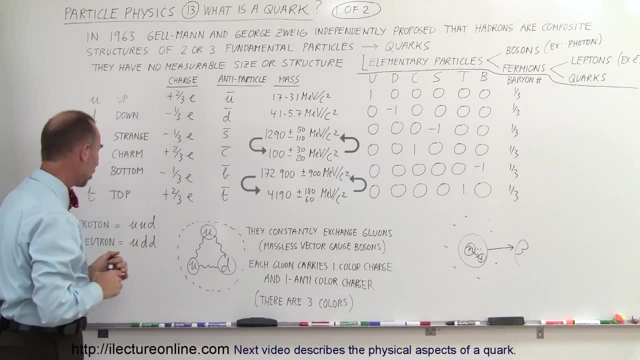 So either a quark had two-thirds of that charge or negative one-third of that charge, And you can see that if you take two up quarks and a down quark together, that would give you a positive one charge. So therefore a proton would then be made up of two up quarks and a down quark, giving it a positive one charge And a neutron would be made up of an up quark and two down quarks, Because one up and two of these would cancel each other out and would be neutral in charge. So it made a lot of sense. 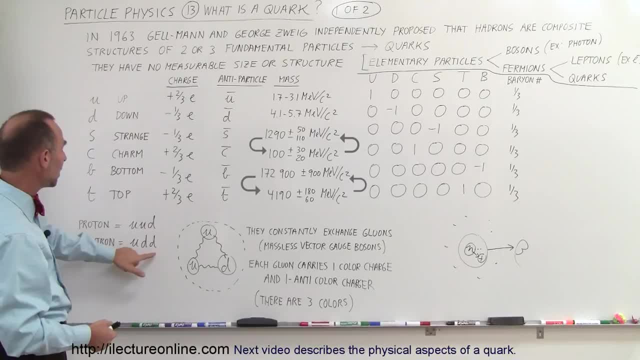 And so then there of course had to be a mechanization that somehow something made up of an up and two down quarks could eject a beta particle, an electron, and turn itself into two ups and a down quark. And so that is something for later. 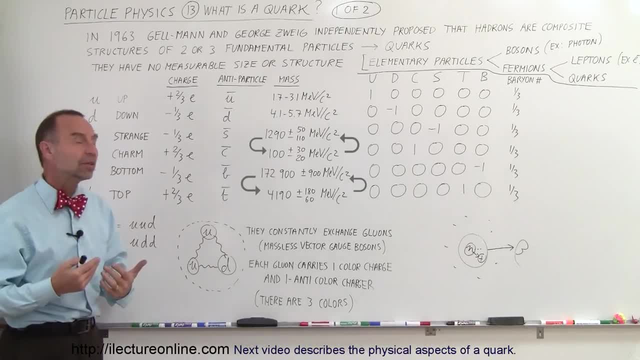 What they also discovered was that, through some experimentation, they actually determined the mass. of course, not back in 1963, but many years later, when they started studying this, They actually realized that there was a certain amount of mass associated with them. 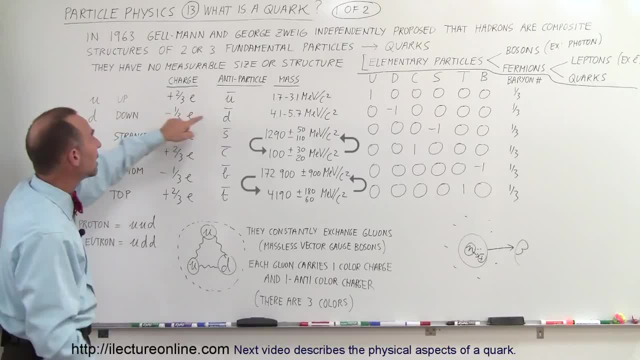 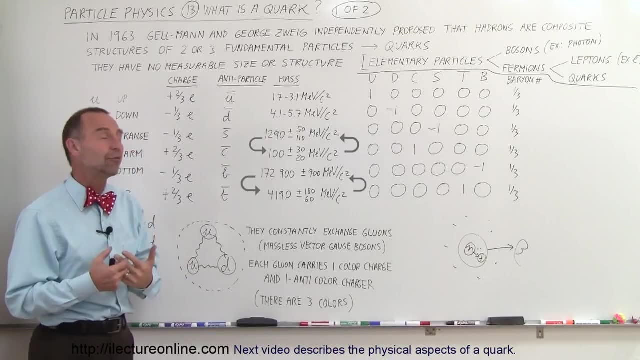 What was really astonishing was that if you, for example, take a look at the mass of an up quark, it's somewhere between 1.7 and 3.1 million electron volts. That would only make it about three to six times the mass of an electron. 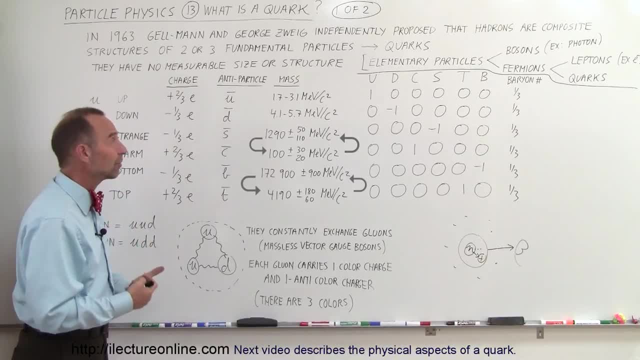 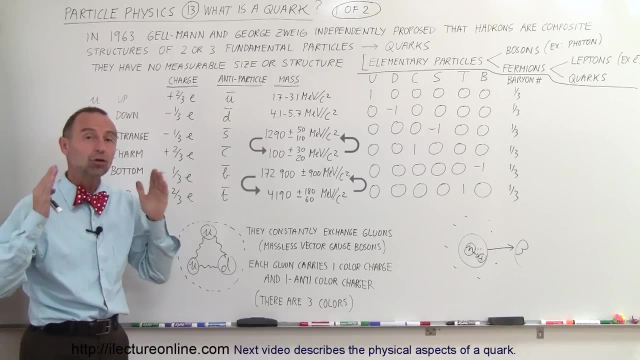 And we know that the mass of a proton is about 2,000 times the mass of an electron. So if you take two up quarks and a down quark, which is about 11 or 12 million electron volts, it falls far short. 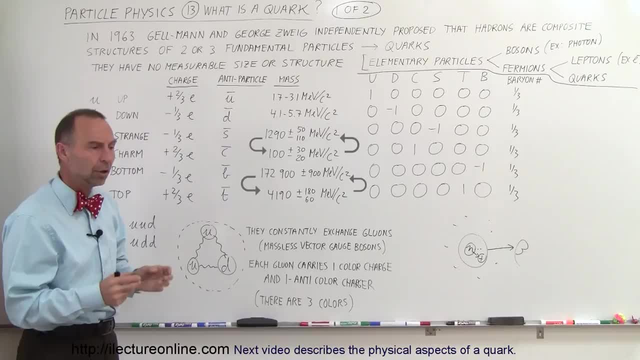 Or the mass of an actual proton, or the mass of a neutron, for that matter. So it seemed like the mass of the quarks was very small compared to the mass of the hadrons that they made. So that was a very big mystery. 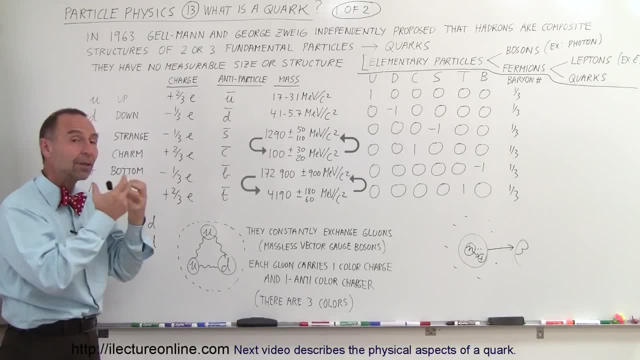 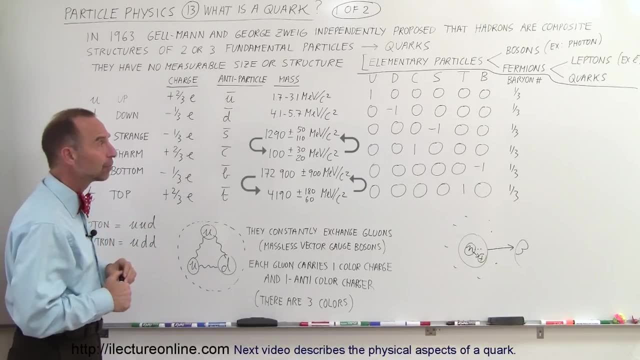 But then, of course, knowing that E equals mc squared, they figured out a lot of the mass would be taken up by the energy that it would contain to hold those quarks together, And that is probably the case. Another thing that they wanted to do is give these quarks some sort of property. 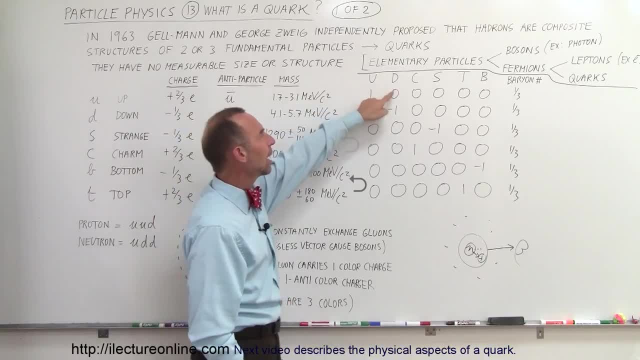 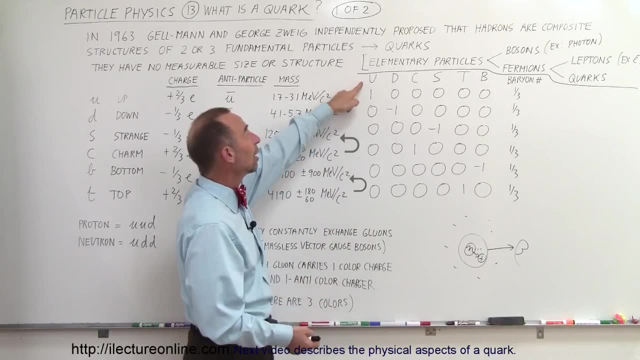 And so it turned out they came up with a six, So six types of properties up down, charm strange top and bottom property, And each would then have an associated property assigned to it, which means the up quark has an up property. 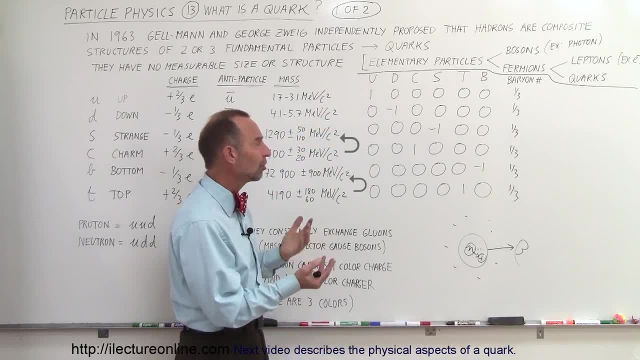 the down quark has a negative one down property and so forth. So they assign plus and minus, and again I'll get to that in a later video. Also, we know that we have a baryon number, so a neutron and a proton has a plus one baryon number. 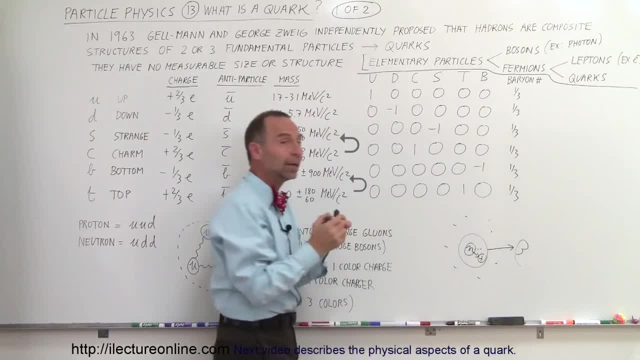 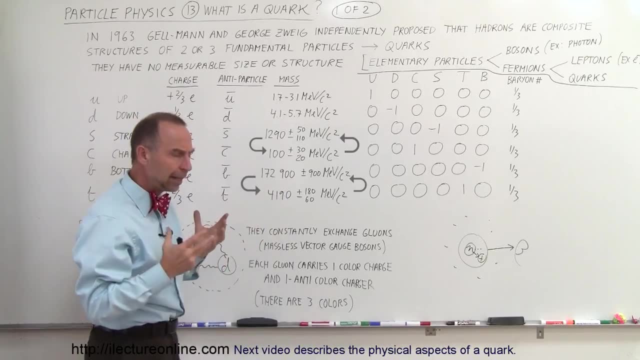 which means, then, that each quark would have one-third of that baryon number three quarks, of course, making up a quark. So we have kind of an idea of how to lay this out. Now we still need to understand a little bit more about how quarks stay inside a nucleon like that. 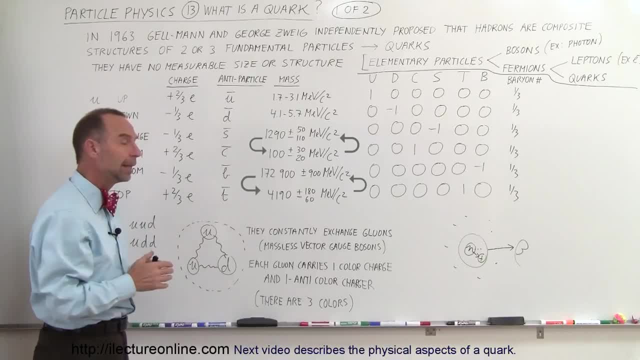 inside a proton or neutron. Why would they do that? What was going on? And so they figured that there was this nuclear strong force holding these together by using an exchange particle constantly going back and forth between the different quarks inside one of those nucleons. 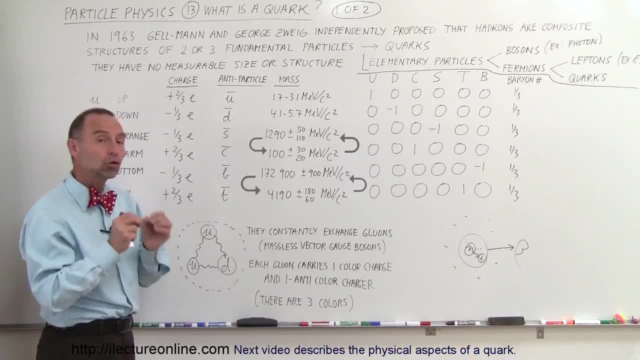 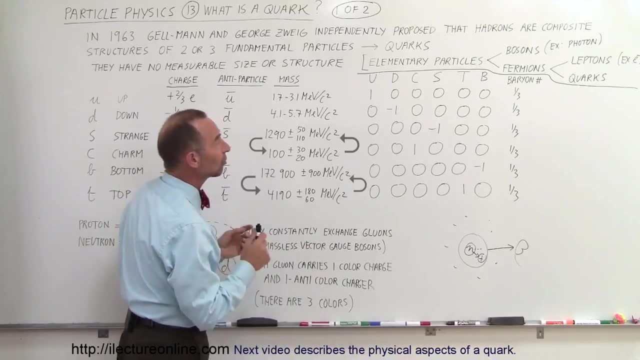 And so the particles being sent around, they end up calling those gluons, And so they're then considered to be massless and they're called vector-gauge bosons. They're part of the boson family, where photons are also part of that family. 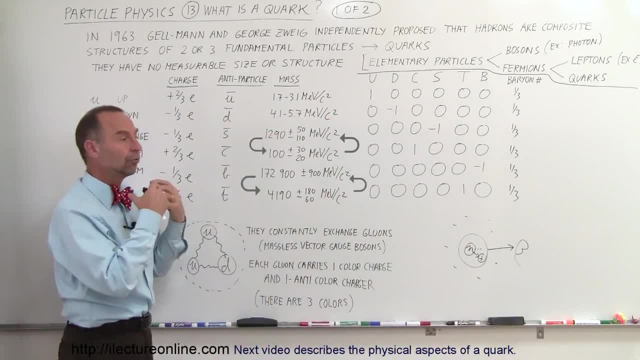 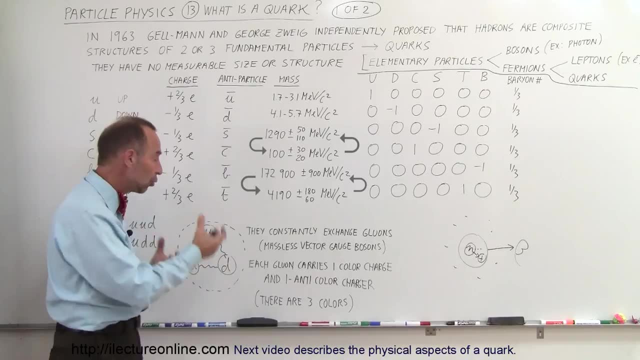 So you can see that photons and gluons have a lot in common. Photons are the exchange particle between the electromagnetic forces, and gluons would then be the exchange particle between the quark forces, the strong forces that keep the quark together. 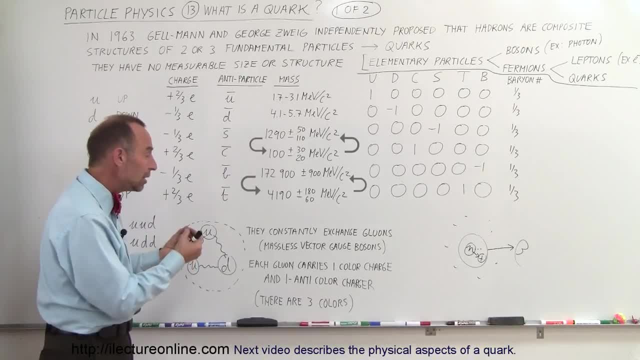 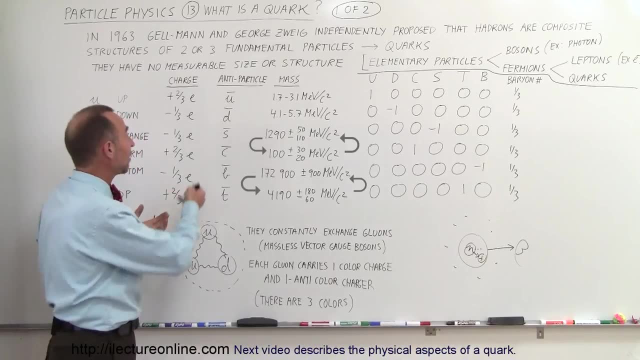 There's some interesting concepts of that, and I'll get into more detail later. What we need to understand, though, is that the quarks also contain another type of charge, So we already know that quarks have either a positive or negative charge. 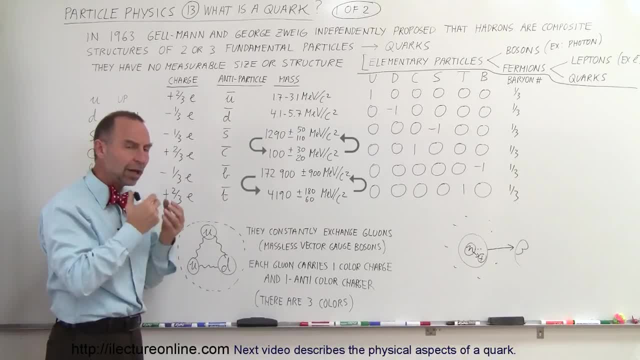 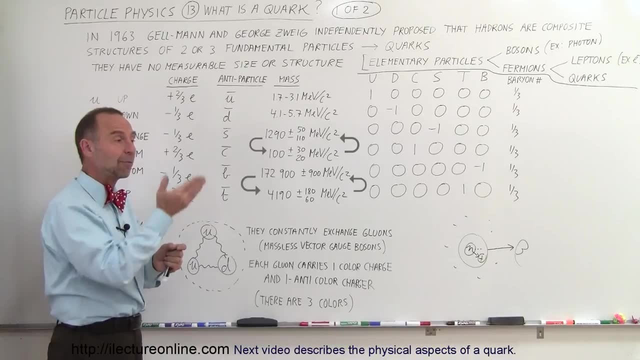 a fraction of an electron charge. But there's another kind of charge, keeping the quarks together. Now it turns out there's more than one charge. For example, we have a positive and negative charge When it comes to these different kind of charges holding the quarks together. 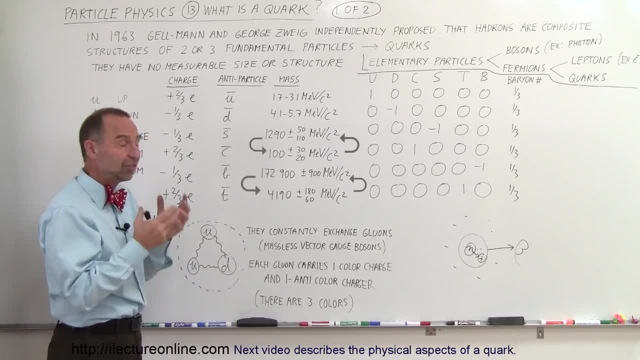 we call them color charges because we didn't have another name for it And since there were three different kinds of charges there, which is strange, we only have a positive and a negative, which is two different kinds. With the quarks there's three different kinds of charges, so we call them color charges. 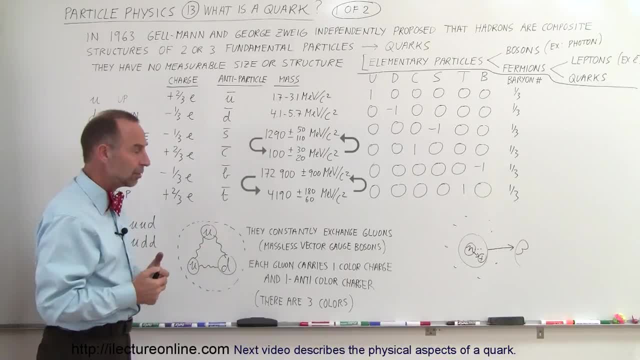 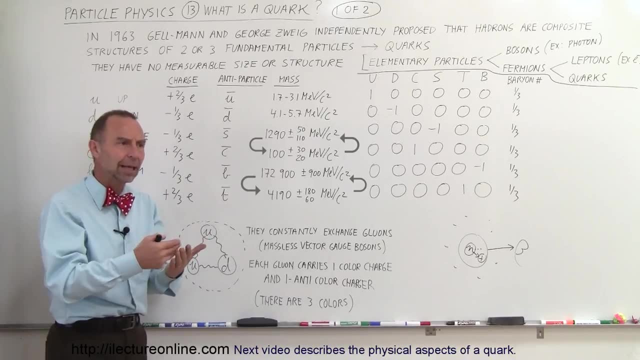 And so we call them blue, red and green. So there's a blue charge, a red charge and a green charge, And it turns out there's an anti-charge as well. There's an anti-blue, an anti-red and an anti-green charge. 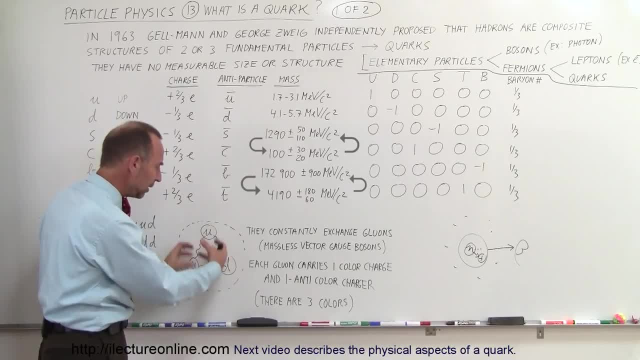 So there's a total of six different charges associated with keeping quarks together inside a nucleus, Or I should say inside a nuclear particle. Not a nucleus but a nuclear particle. And so it turns out then, when gluons are going back and forth, holding these together. 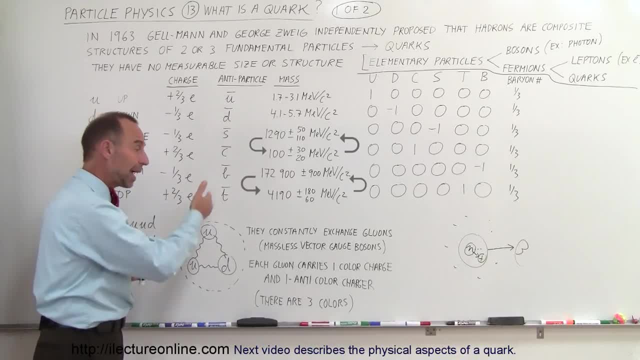 each gluon carries one of the colors and one of the anti-colors back and forth, And when a gluon moves from one quark to another it takes away color and so it changes the color charge of the quark, as the gluons are constantly going back and forth. 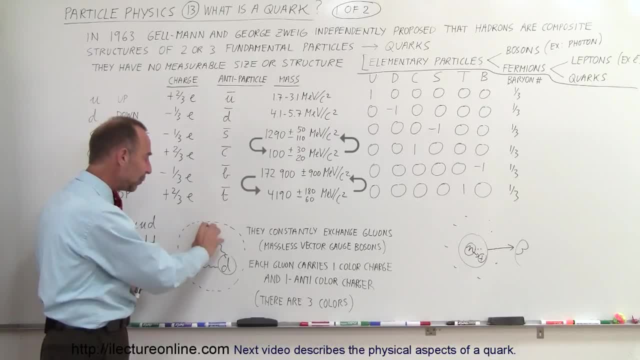 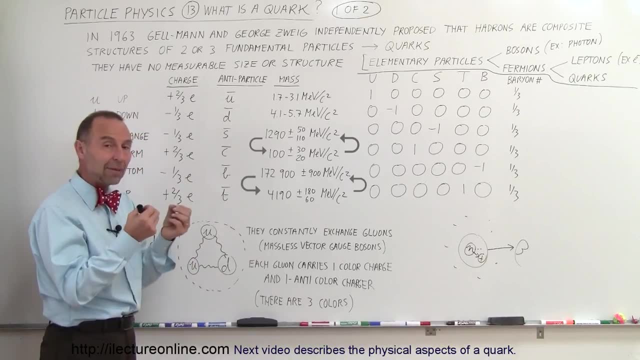 So the color charges are constantly changing with these quarks inside the proton or neutron. And what's interesting is we realize that if the the colors are the same, if two quarks have a red charge, they will repel each other. If they have a different charge, they will attract each other. 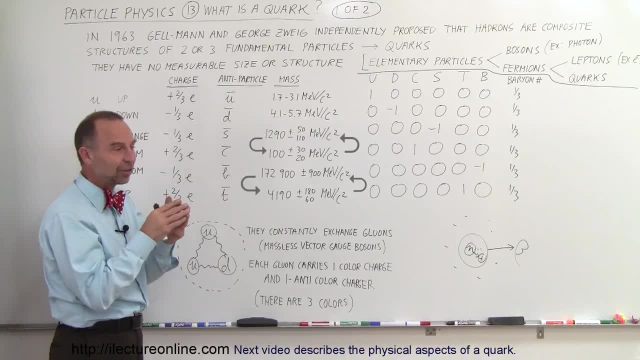 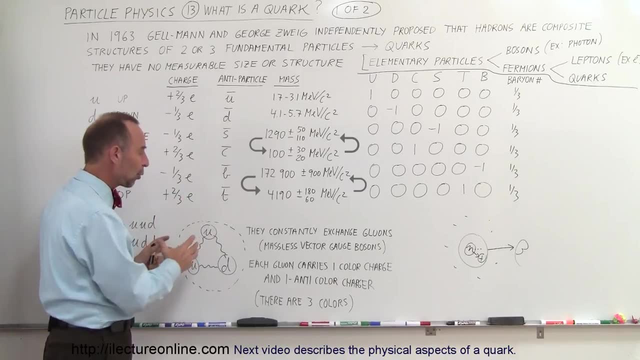 So we have three different colors and three different anti-colors. and the three colors: if they're different, they attract, If they're the same, they repel. What's also very interesting about the quarks is that the amount of force between them increases.